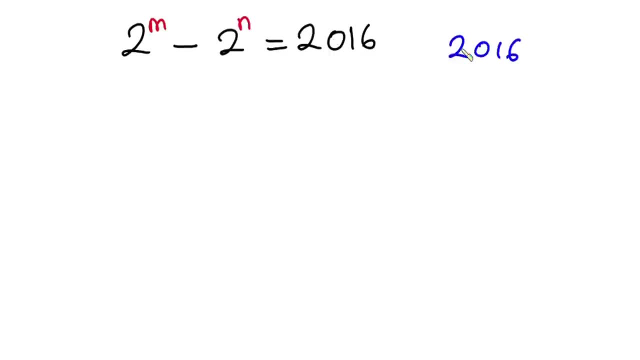 have 2016 over here. this is a positive number, meaning that it is greater than zero. so if 2016 is greater than zero, then let's consider the left hand side over here. so this means that two to the power m is greater than two to the power m. 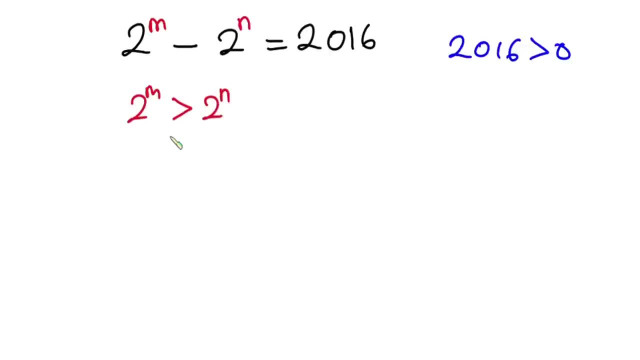 okay, the bases are the same. so it means that m is greater than n, do you agree? all right, so here we can say that m is greater than n. now, under what instance can we make m equal to n? well, we can say that m is equal to n when we add a certain variable, say k to n, or n will be equal to m. 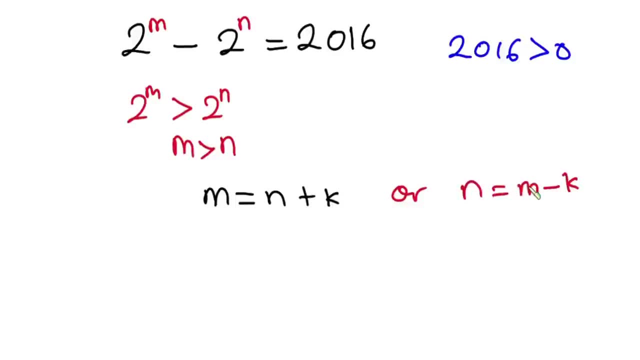 when a certain constant, say k, is subtracted from m. do you agree? but you focus on this one. okay, so now we have: m is equal to n plus k. so in place of m, i'm gonna put n plus k in this equation. so we have two to the power n plus k minus two to the power n is equal to 2016.. all right, so here. 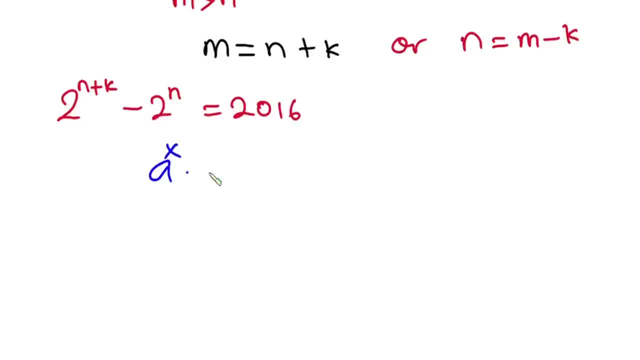 if you have a to the power x times a to the power y, this could be written as a to the power x plus y. so we have two to the power n times two to the power k minus two to the power n is equal to 2016.. 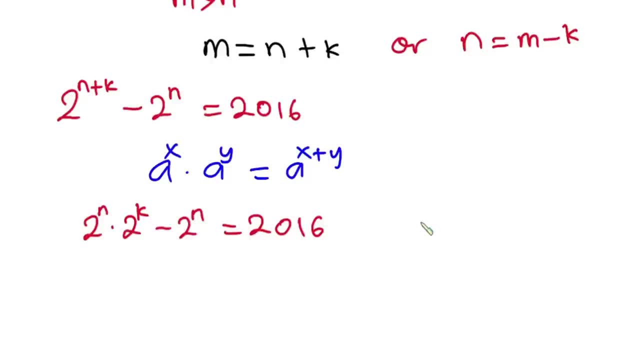 all, right now let's express 2016 in a form that will get two to the power. let's say d in it. okay, so 2016 is the same as 32 times 63, and 32 is two to the power. five then times 63. so we can express 2016 in the form of this. so, in place of 2016, we'll put this one there. 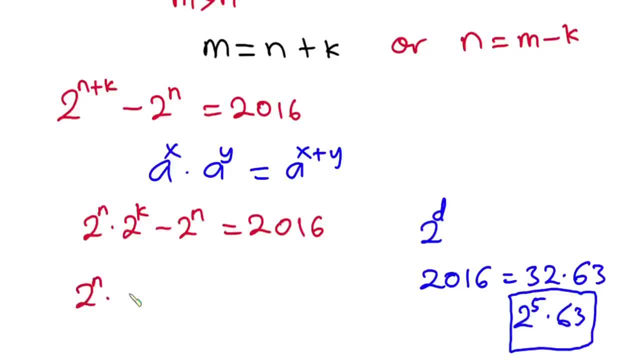 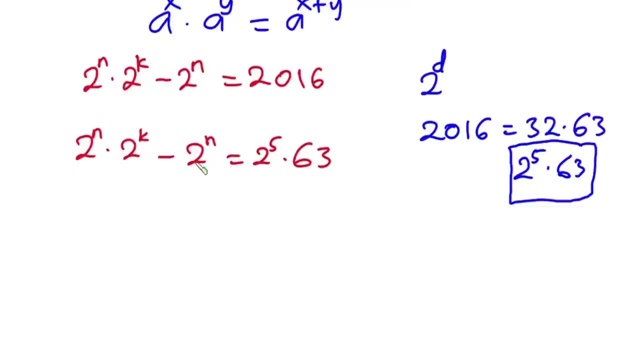 so we have two to the power n times two to the power k minus two to the power n is equal to two to the power five times 63. all right, so here we have two to the power n here and then two to the power n, so we can factor two to the power and out. so we have two to the power. 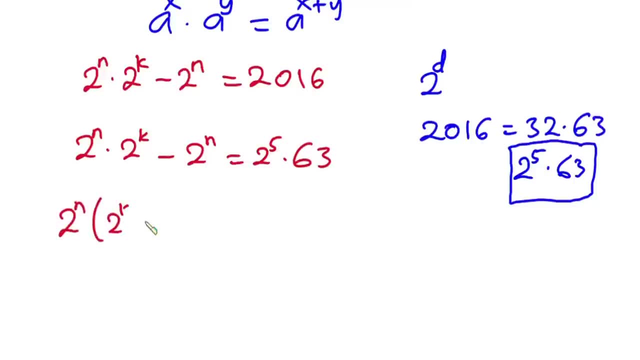 n into two to the power. k minus one is equal to two to the power five times sixty three. all right, now let's consider this two to the power end. here is an even okay so example. when 2 is raised to a fourth power, this is equal to 16, where 16 is an even number. 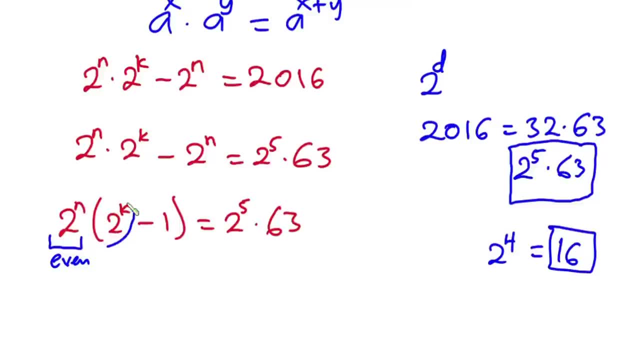 then let's consider this one: 2 to the power k is also an even number, but when we take one from it, the whole of this one becomes an odd number. okay, now let's consider this side. 2 to the power 5 is also an even number. all right, then. 63, as you all know, is an odd number. all right, so now let's. 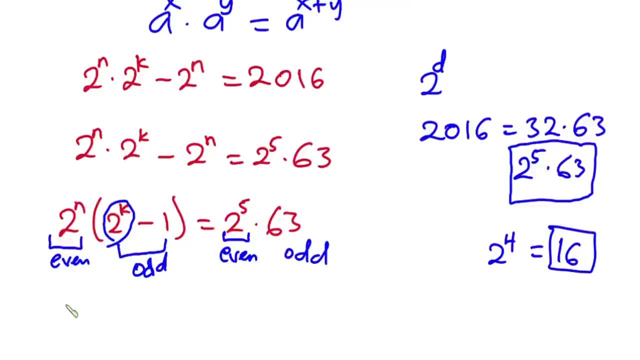 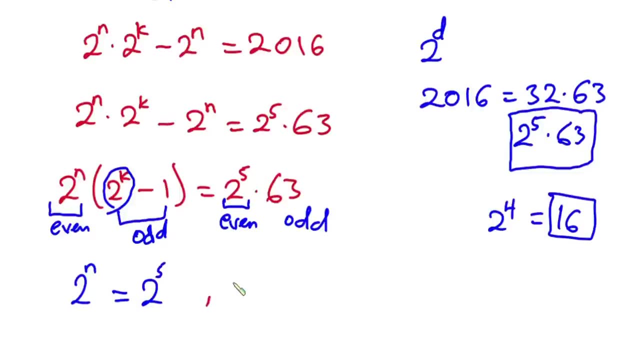 compare even to even and then all to all. now we have 2 to the power- n is equal to 2 to the power 5, and then 2 to the power. k minus 1 is equal to 63. all right, so now let's find this 2 to the power. 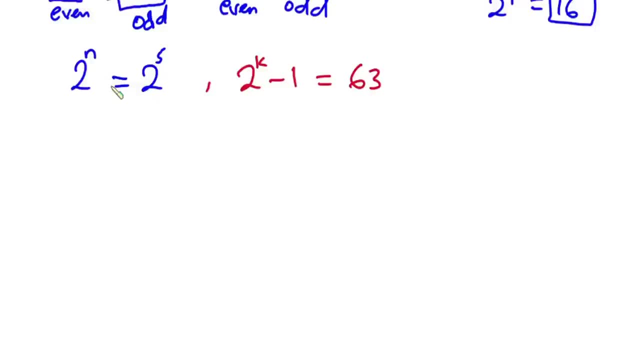 n is equal to 63, all right, so now let's find this: 2 to the power n is equal to 63, all right, so now let's find this: 2 to the power n is equal to 2 to the power 5. the bases are the same, so we can. 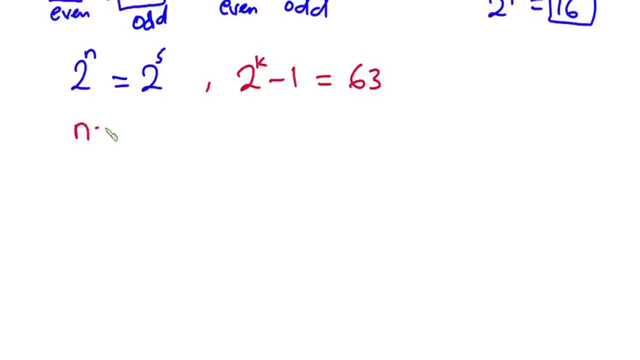 equate the exponent. so this means that n is equal to 5. now let's focus on this equation from here. we can say that 2 to the power k is equal to 63 plus 1. all right, so we have 2 to the power k. 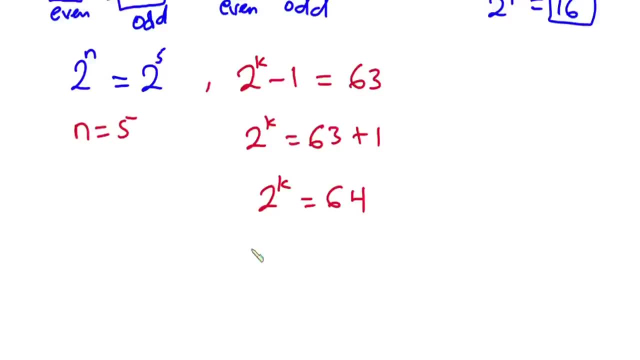 is equal to 64. now we have 2 to the power. k is equal to 64 could be written as 2 to the power 6. all right, now, since the bases are the same, we can easily equate the exponents. so we have: k is equal to 6. now we know that n is equal to 5, k is equal to 6, but we don't know m. all right. 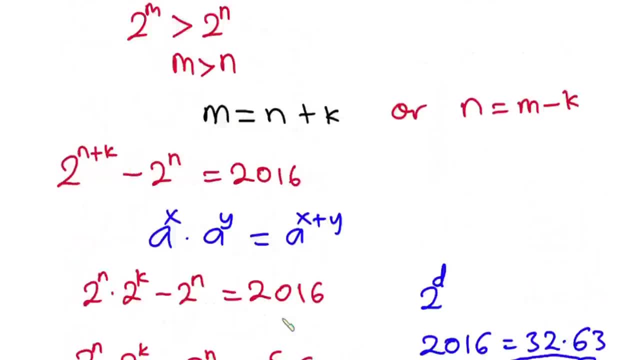 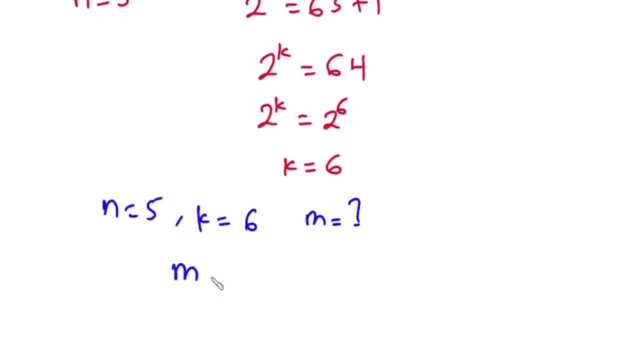 so now let's find m. we know that m from here is equal to n plus k, so we can say that n is equal to n. where n is 5, then plus 7, and we know that n is equal to 6, so we know that n is. 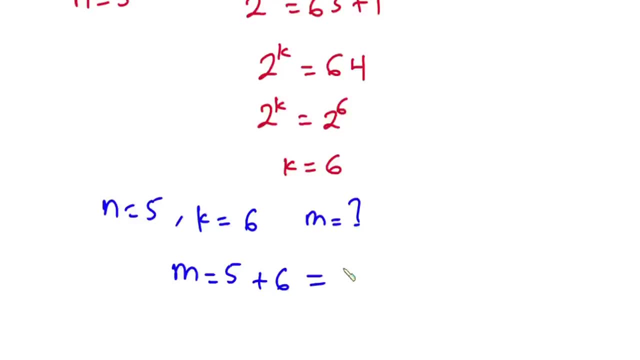 k, where k is 6, and this is equal to 11. so therefore we can say that m is equal to 11. all right, so now we know that m is equal to 11 and then n is equal to 5. so, guys, i hope you enjoyed. 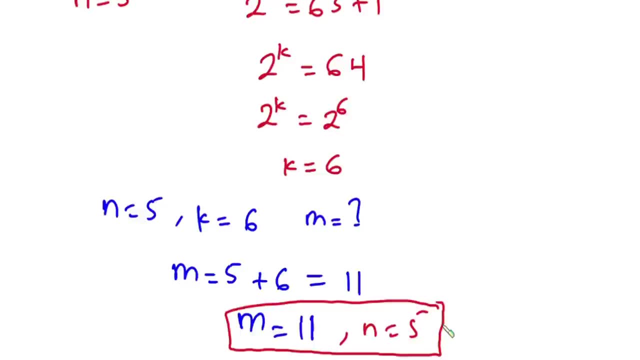 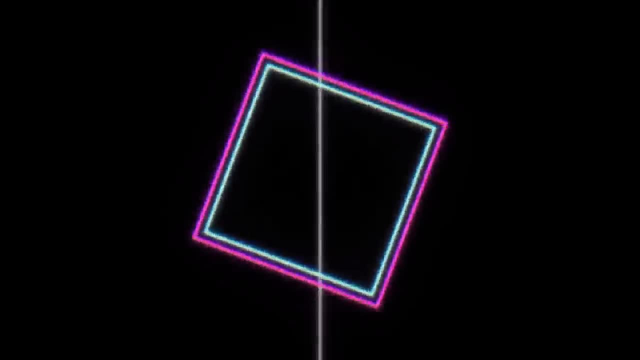 watching this video. please give it a thumbs up and also don't forget to subscribe to this channel. thanks a lot for watching. see you again on the next video. you. 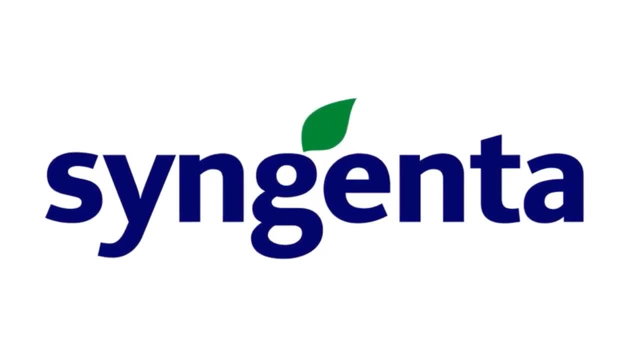 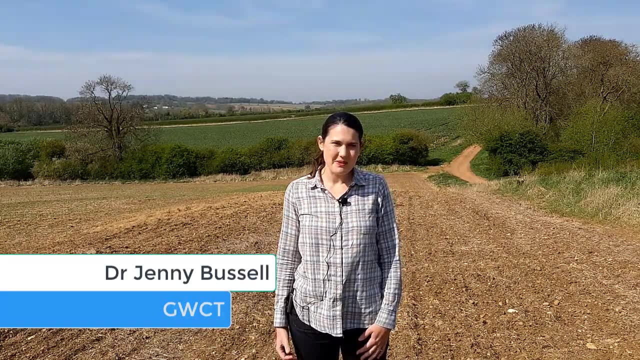 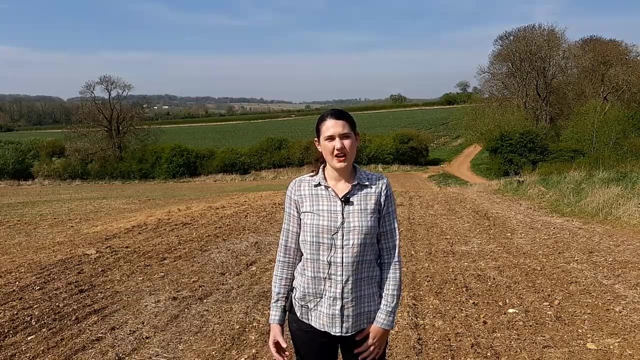 So at Luddington we've been measuring soil health by looking at things like earthworm numbers. Earthworms are key indicator species and generally when earthworm numbers are high in your fields it means you've got high soil activity and good soil health. 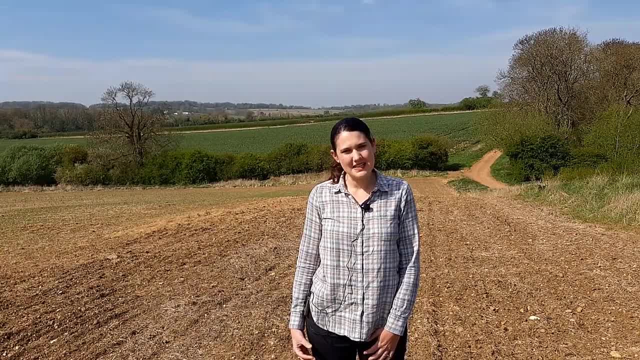 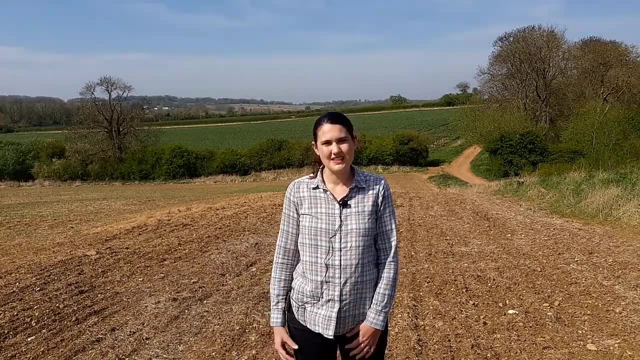 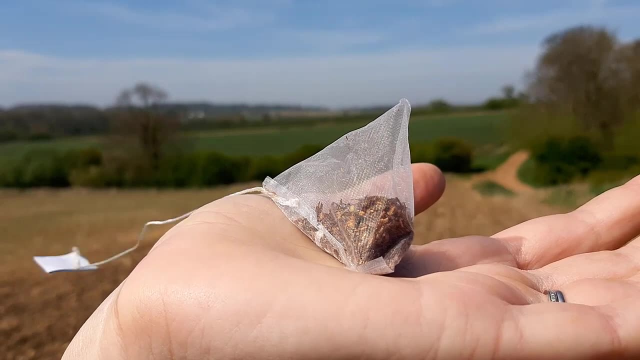 We've also been looking at visible assessment of soil health- so digging up the soil and looking at its colour and its structure to help us see whether there's improvements in soil health when we change some soil management- And we've been pairing teabags to look at both soil activity and soil organic matter stability. 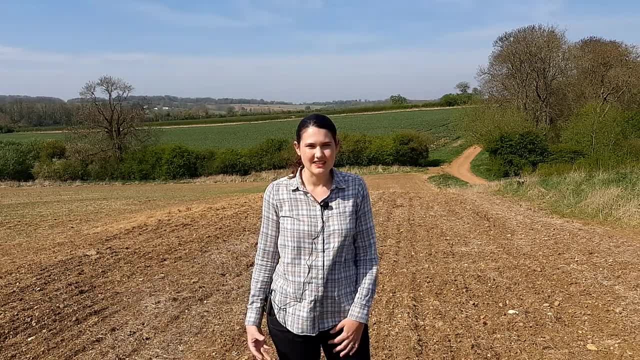 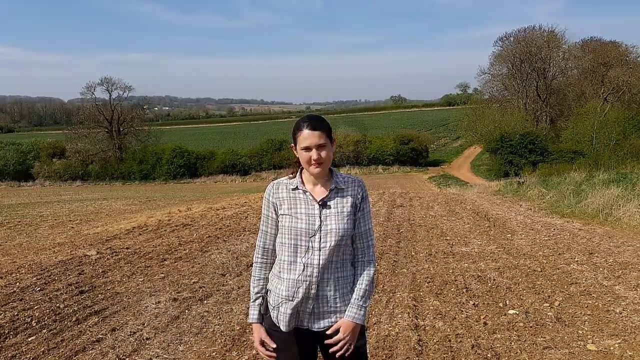 so how much soil organic matter is being cycled in through your soil, but also how much is being stored and kept there in order to improve the soil organic matter within the soil With worms? we've found that the numbers have increased in their minimum tillage plots.